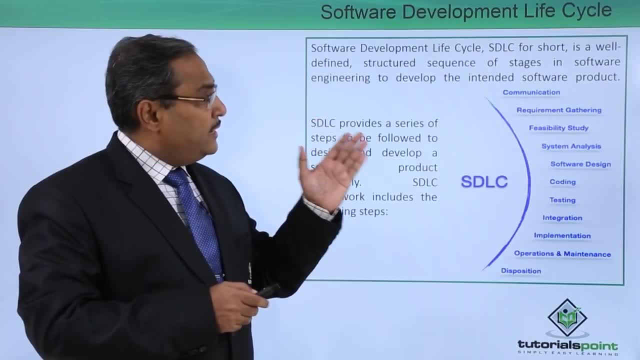 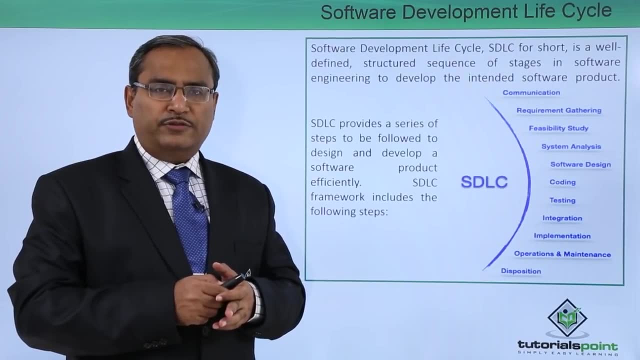 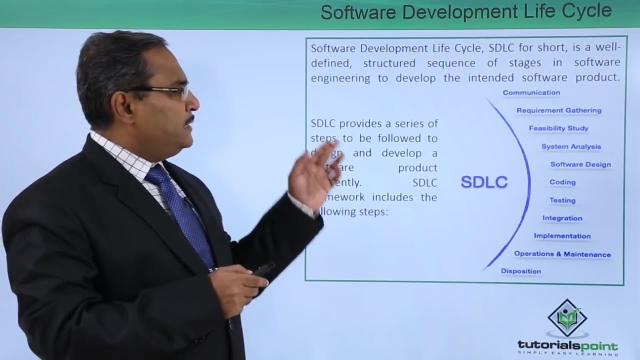 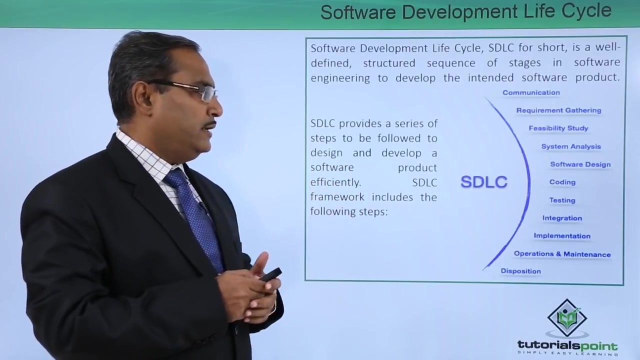 defined structured sequence of stages in software engineering to develop the intended software product. We know that whenever we develop one software for a specific application, then usually we call it as a software product. So SDLC provides a series of steps to be followed up and to design and develop a software product efficiently. SDLC framework includes: 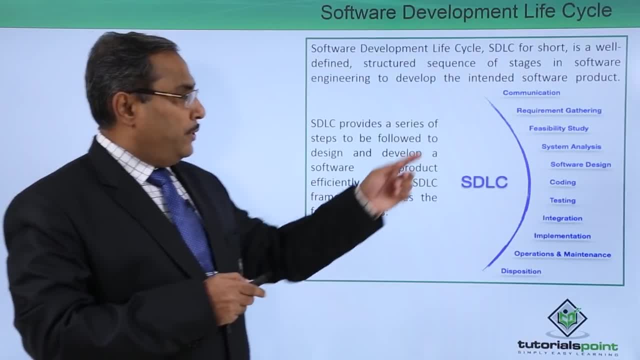 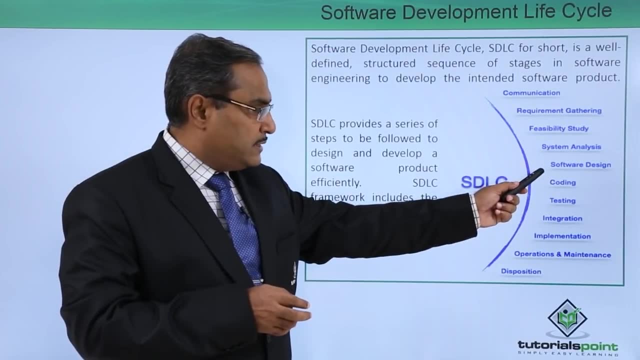 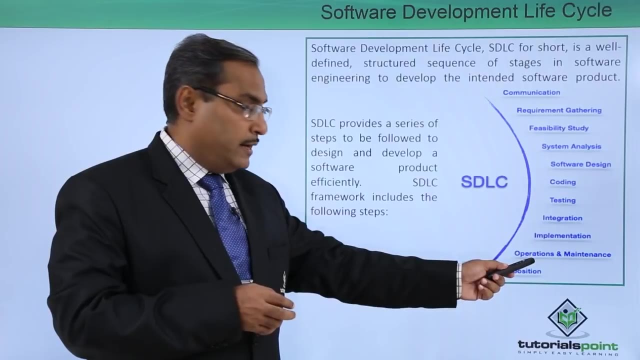 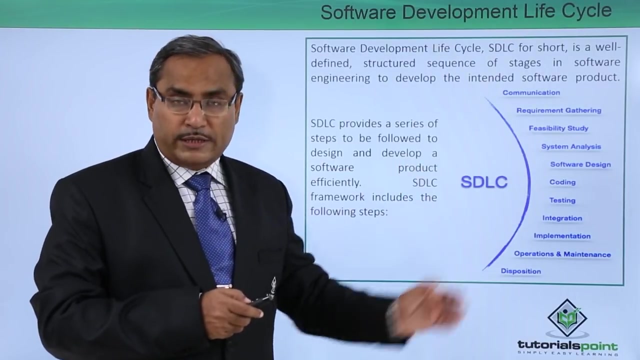 the following steps. So what are the steps we are having? We are having communication, requirement gathering, feasibility study system analysis system, software design, coding, testing, integration, implementation, operations and maintenance, and here we are having disposition. So these are the different phases or stages through which the SDLC is to take place. So 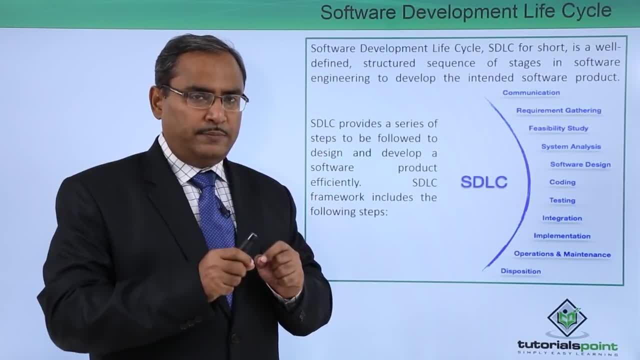 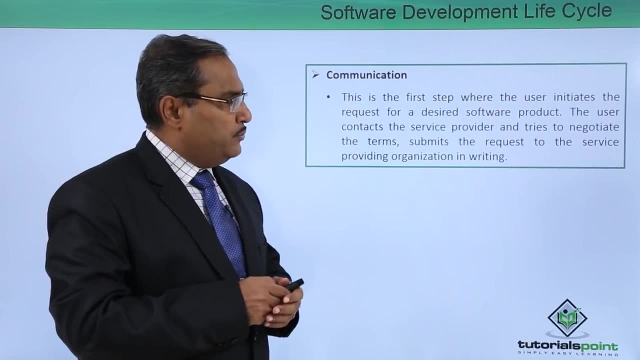 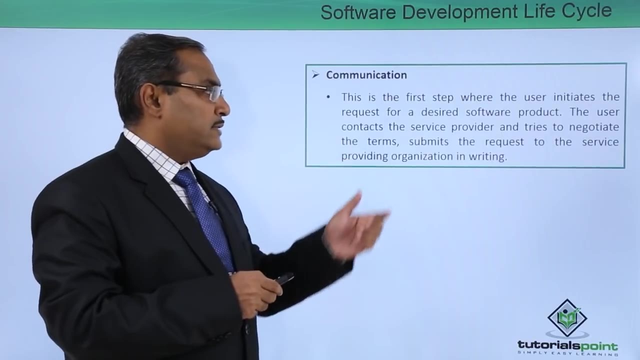 let us go one by one. We shall discuss Each one of them into further details. So at first we are sticking with the communication. This is the first step, where the user initiates the request for a desired software product. The user contacts the service provider and tries to negotiate the terms. submits a request. 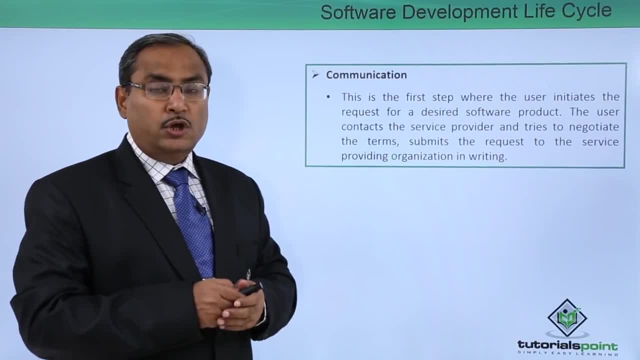 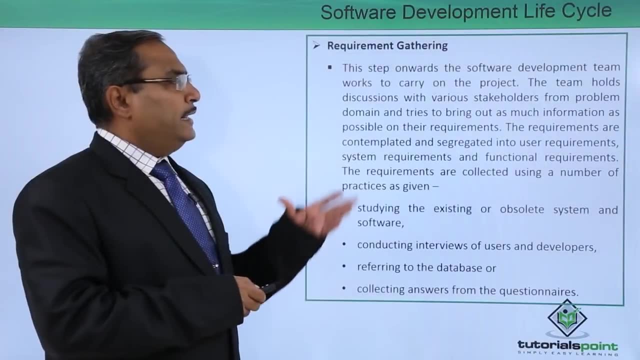 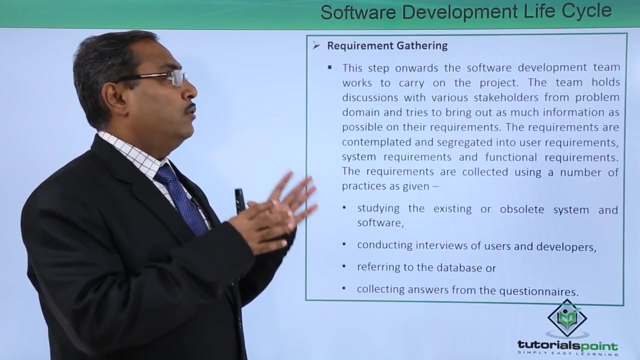 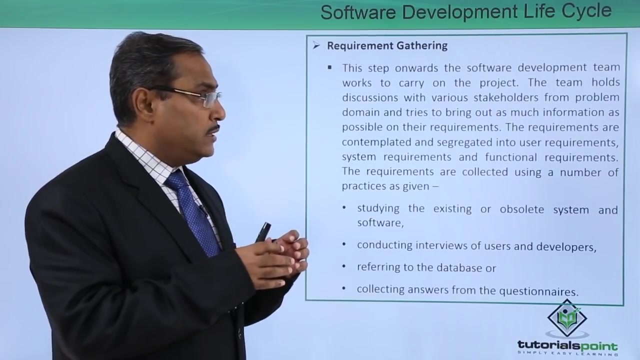 to the service providing organization in writing. So at first the communication will be built in between the users and the respective service providers. The next step is our requirement gathering. This step onwards, the software developers team work to carry out on the project. So this team holds discussion with various stakeholders. 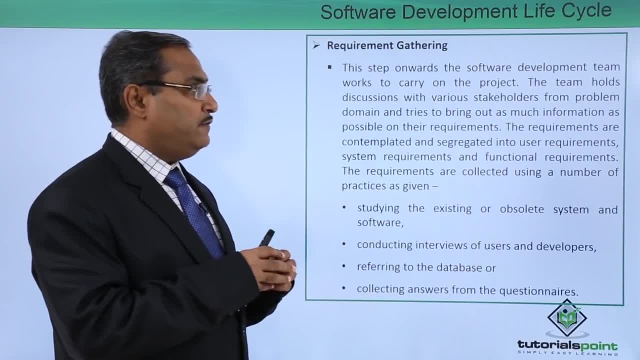 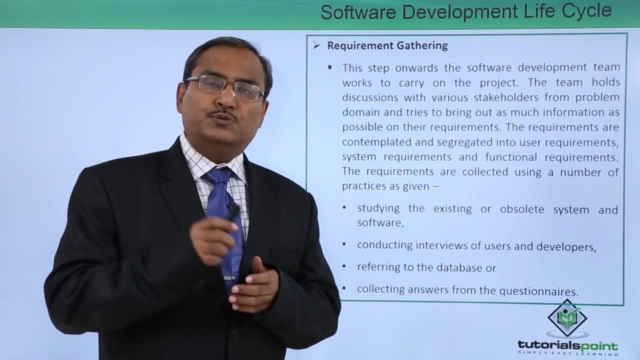 from the problem domain and tries to bring out as much information as possible on their requirements and expectations. So we know that stakeholders are those persons who are positively or negatively affected by the execution of the project. So we know that the staff of the department are those persons who are in the most sensitive position of 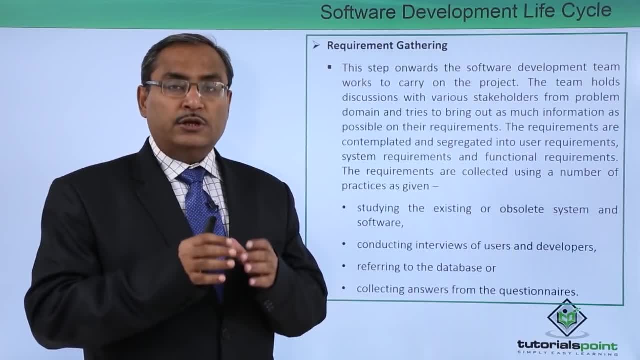 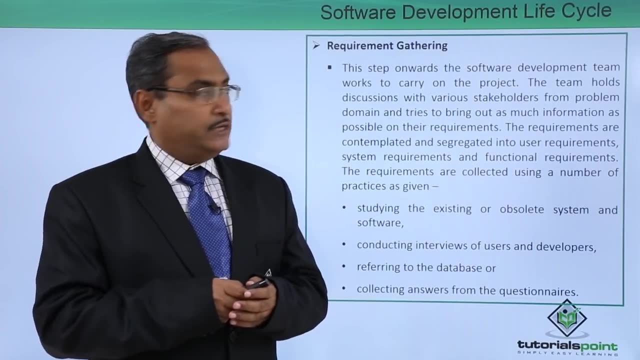 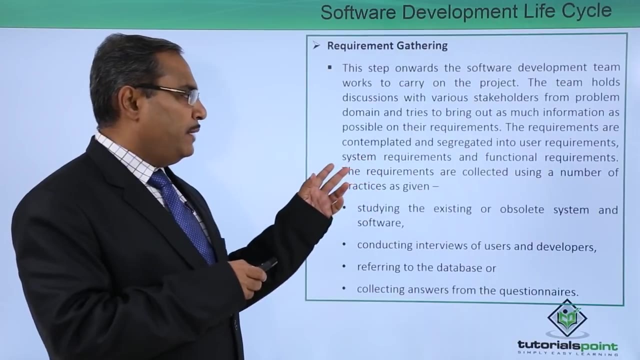 the project. But here we are considering those stakeholders who are from the problem domain so that, after having a good communication with them, we can gather and accumulate all the requirements and their expectations. The requirements are contemplated and segregated into user requirements, system requirements and functional requirements. 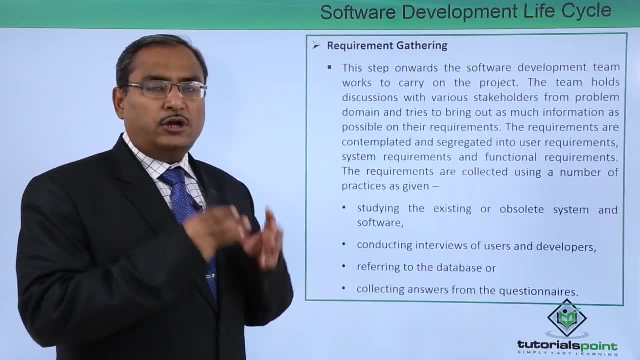 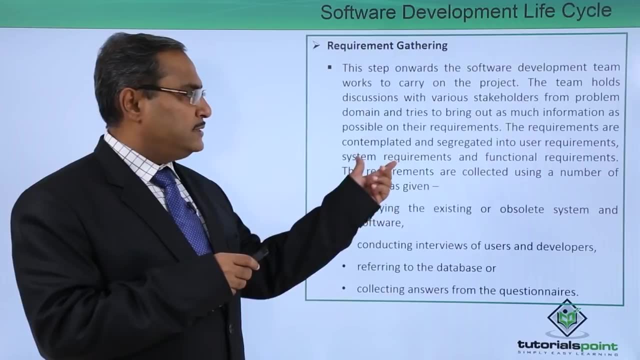 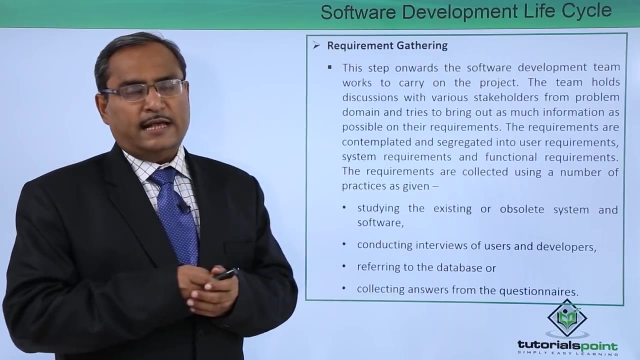 So actually here, after getting all these requirements, the requirements are to be segregated mainly into three different categories. So one is our user requirements. next one is the system requirements and the functional requirements. These requirements are collected using a number of practices, as given. So how can we collect all these requirements from the users? So 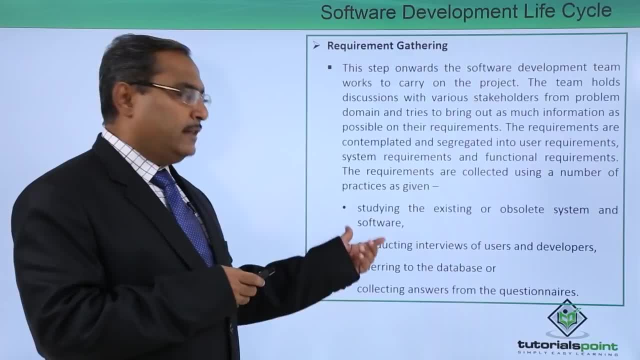 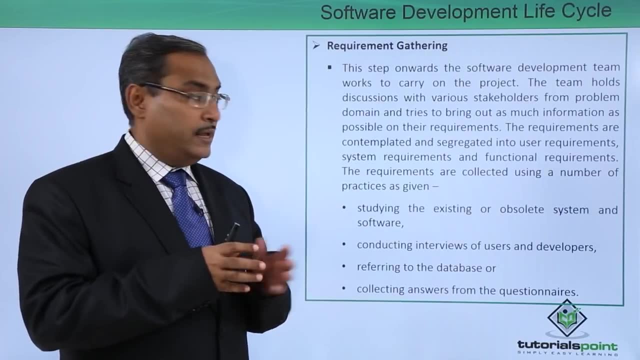 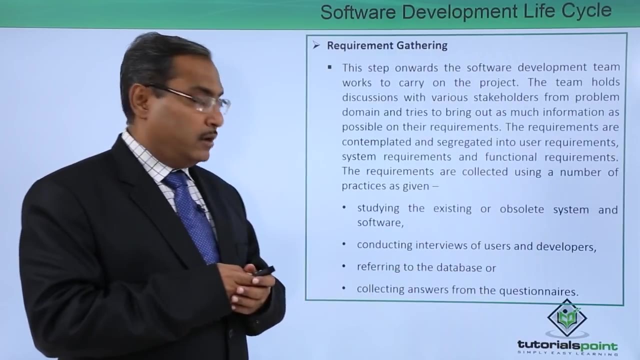 studying the existing or obsolete system and the software. So after doing the study on the existing system or the obsolete system, that means the old version system, and then from there we can easily gather the requirement list. So conducting interviews of users and developers, referring to the databases or collecting answers. 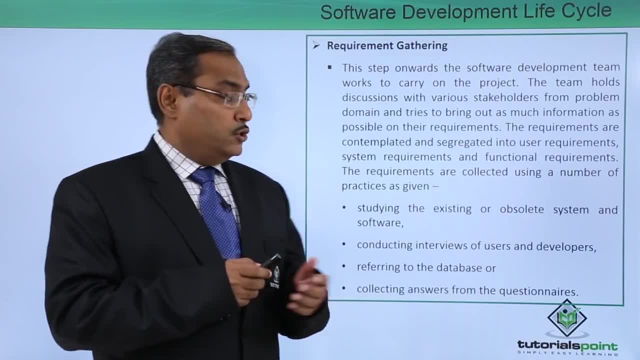 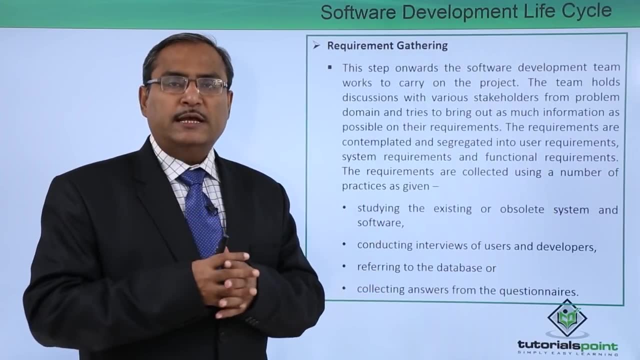 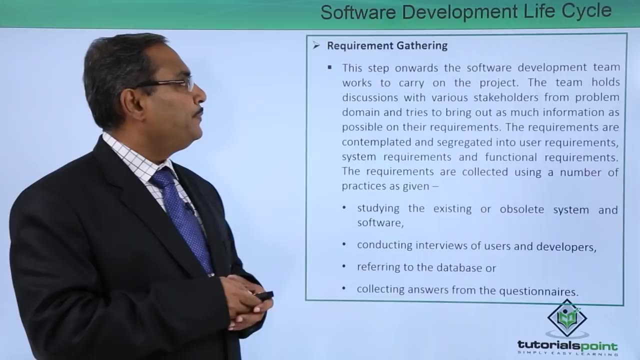 from the questionnaires in the form of a feedback. So, using any one of the methods or combination of multiple such methods, we can gather the requirements and user expectations from the new version of the software or from the newly built developed software. So here we are having one project charter. This project charter may have different formats. 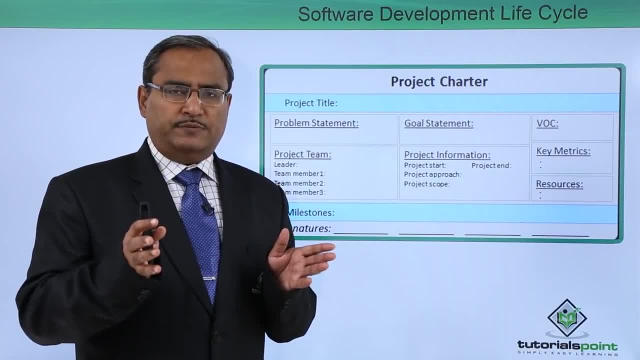 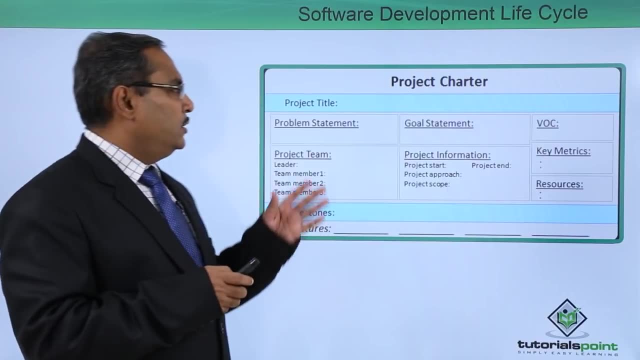 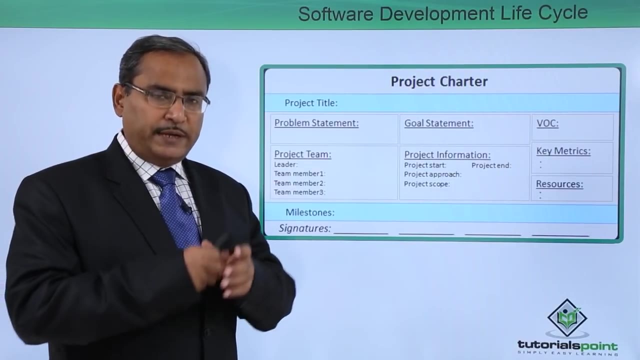 depending upon the company, depending upon the nature of the software project, this project charter fields may get changed. Here we have shown a sample project charter. So it should have a project title, obviously. So on which project title this project charter has been? 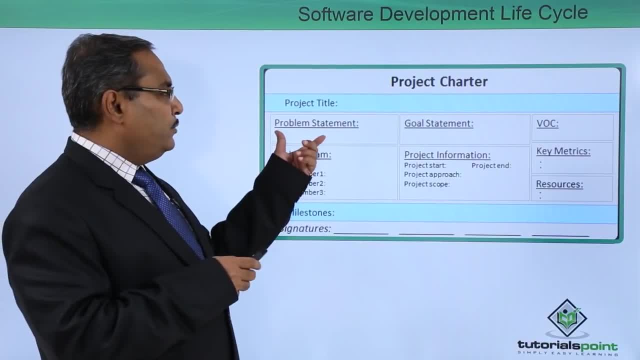 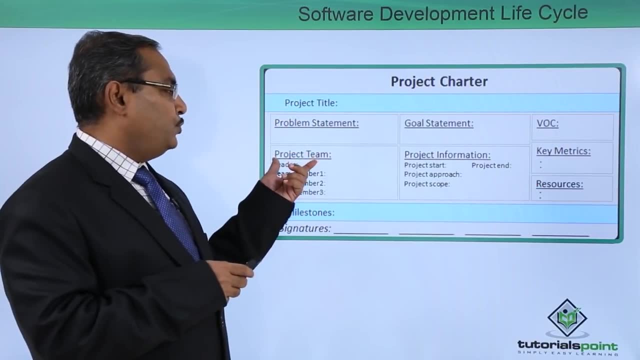 developed. So project title should be there. and then we are having this problem statement, goal statement, the voice of customer. We are having the project team, who is the leader and who are the other team members, member 1,, member 2,, member 3. in this way, We are 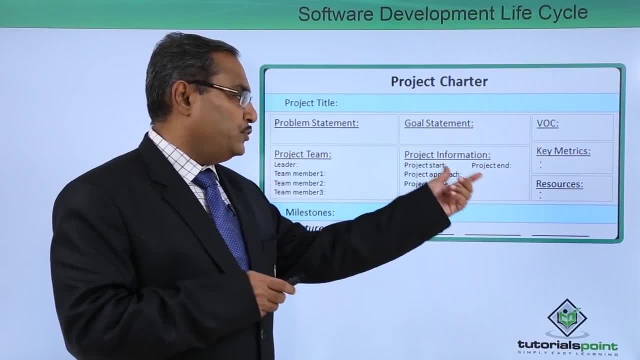 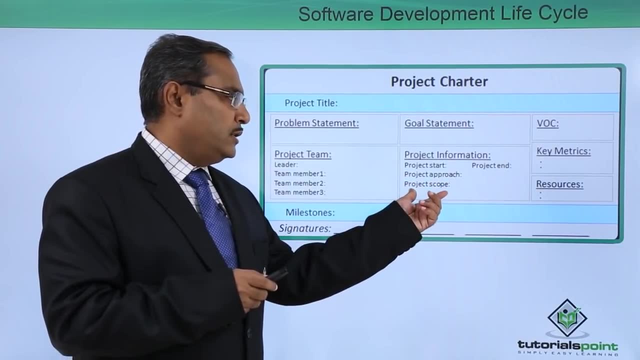 having the project information. there is a project start and project end. A project cannot go forever. it must have a certain start date and end date and project approach, the project scope. what are the features to be implemented? We are having the resources, the key metrics. 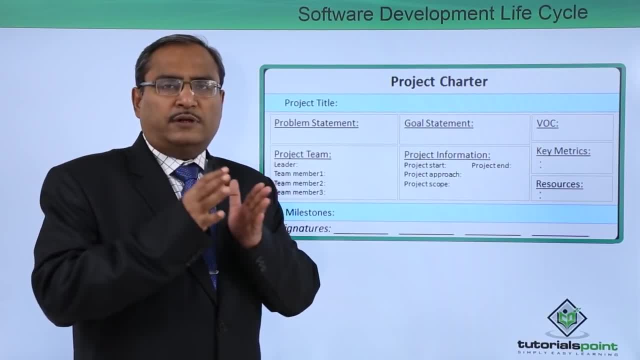 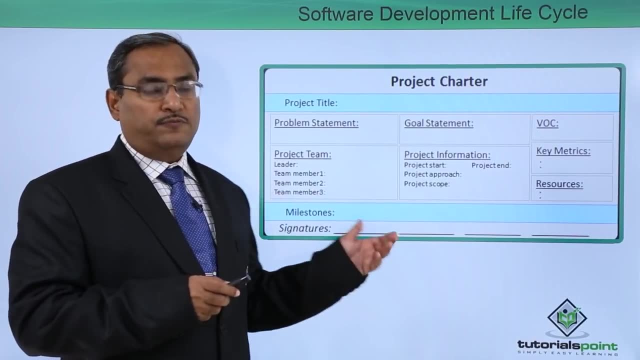 In this way we are having the milestones. that means the how to implement the project. This is how many phases. for the phase segregation, we can put some milestones in between and then the signatures will be there. So for that, some space will be kept. So this is. 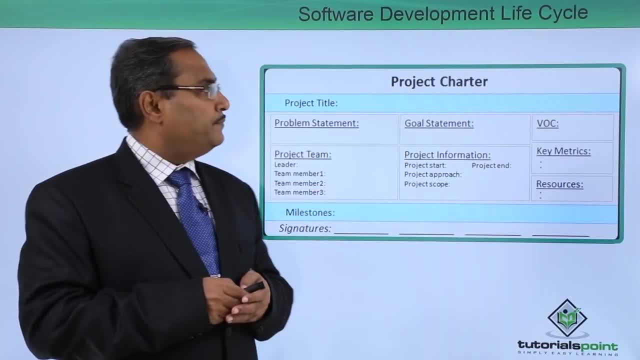 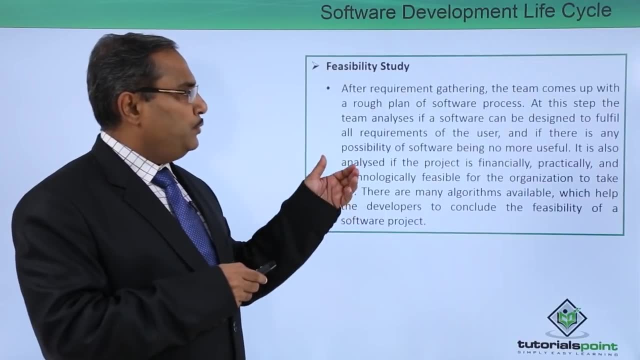 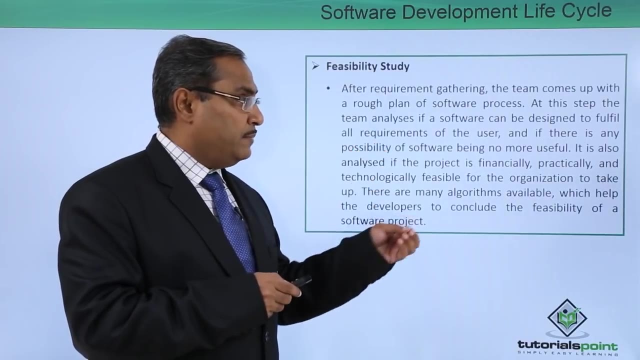 one sample project charter template for your understanding. So next one: we are going for the feasibility study. After requirement gathering, the team comes up with the rough plan of software process. As this step, the team analyzes if a software can be designed to fulfill the required requirements. So the team comes up with the rough plan of. software process. As this step, the team analyzes if a software can be designed to fulfill the required requirements. So the team comes up with the rough plan of software process, Which of all required requirement classes. So that is how we are compound, process the process. 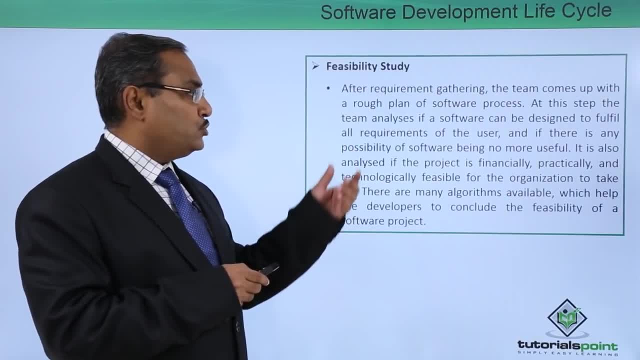 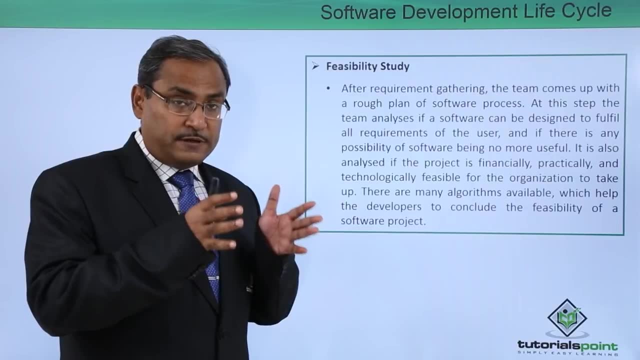 that we are conducting using долларов. So if the project starts with the style of supporting the project right from theiful, engineering all requirements of the user and if there is any possibility of software being no more useful. So in this way we are at first we 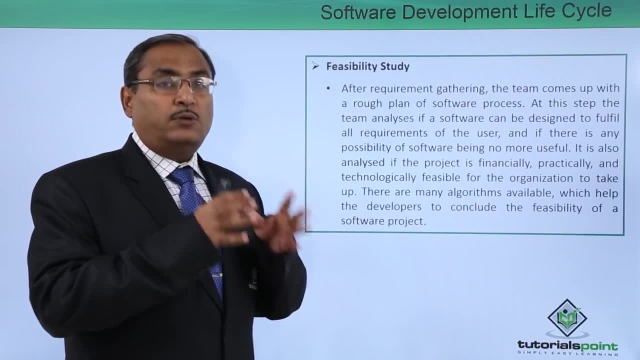 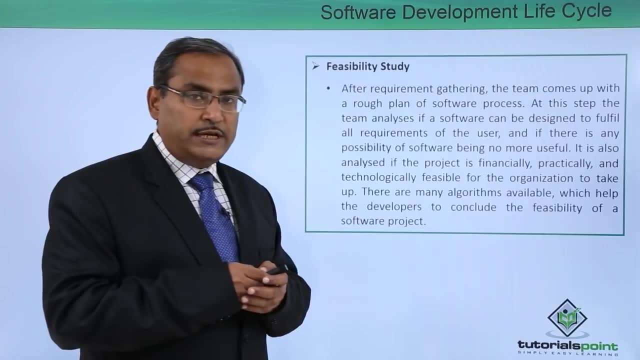 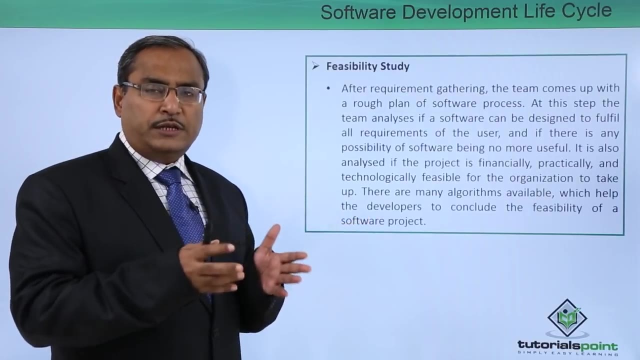 are analyzing all these requirements and you are trying to frame that what software will be the suitable one for this one? It is also analyzed if the project is financially, practically and technologically feasible for the organization to take up. So obviously, whenever you get to a project, you have already developed the planning tools. This is not. 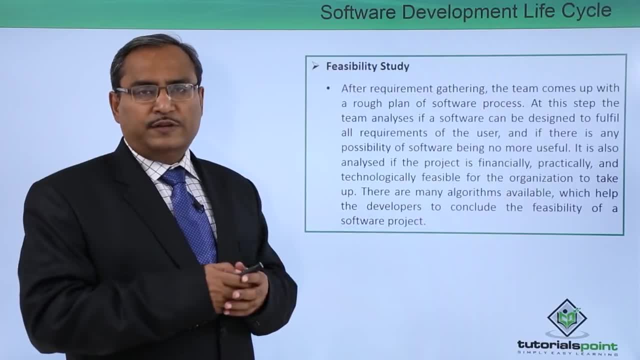 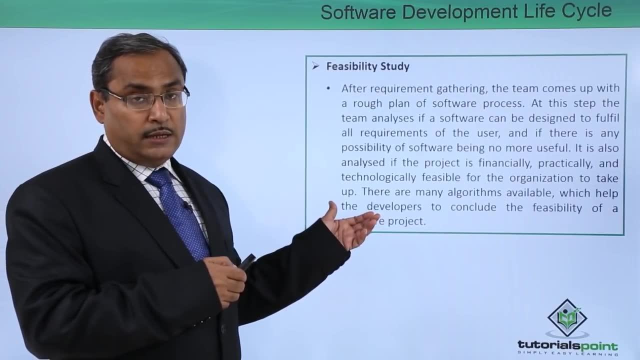 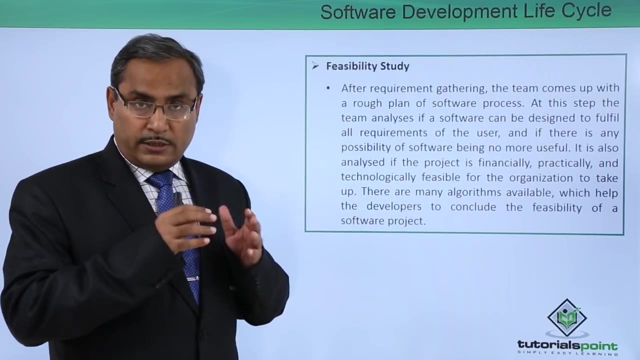 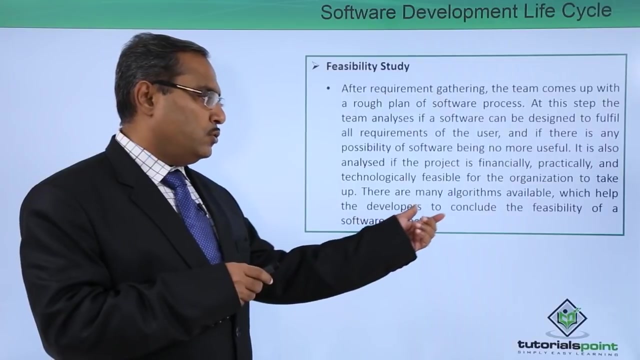 you are going for a very complicated project or very large project, obviously the budget against that project, the cost against that project, will be also high. so whether this company is can permit that that cost, whether this particular organization can take up those challenges. so these things are to be justified. so there are many algorithms available which help the developers. to conclude, 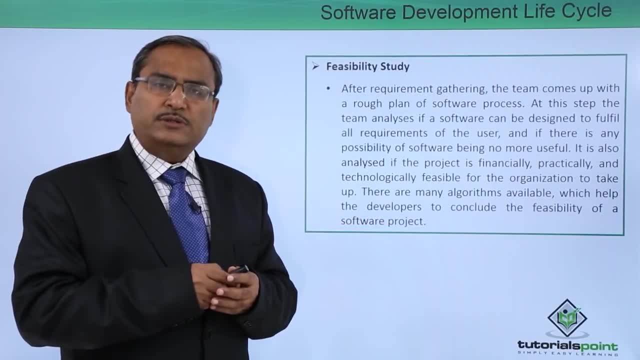 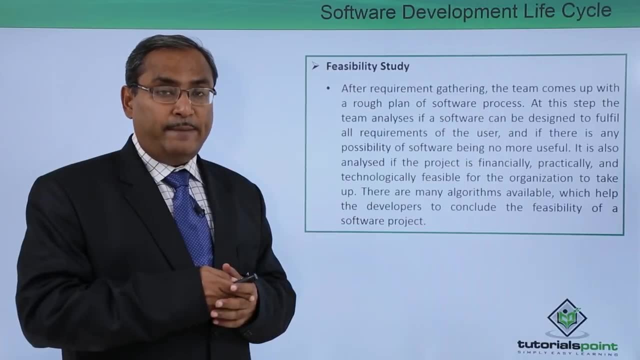 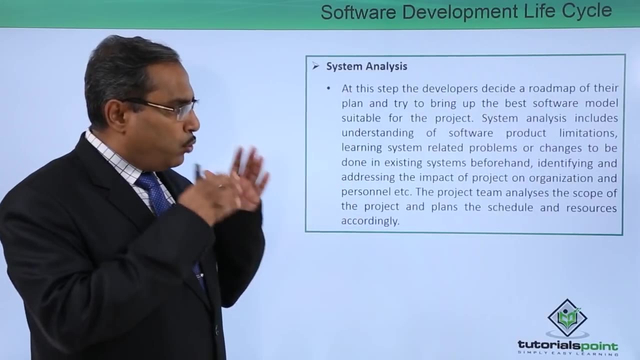 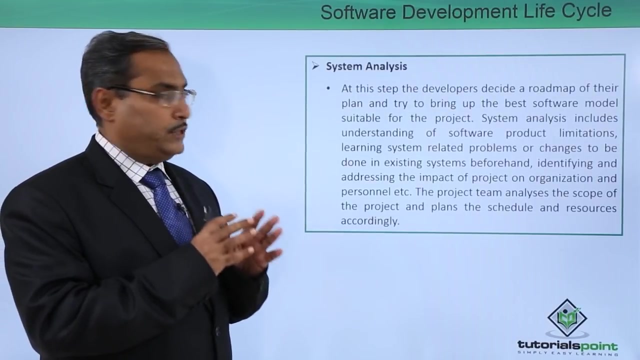 the feasibility of a software projects. so, using different kinds of algorithms, we can test the feasibility of the software project, that how this project can get implemented. so next one: we are having this system analysis. at this step the developers decide a roadmap of their plan and try to bring up the best software model suitable for the project and system analysis. 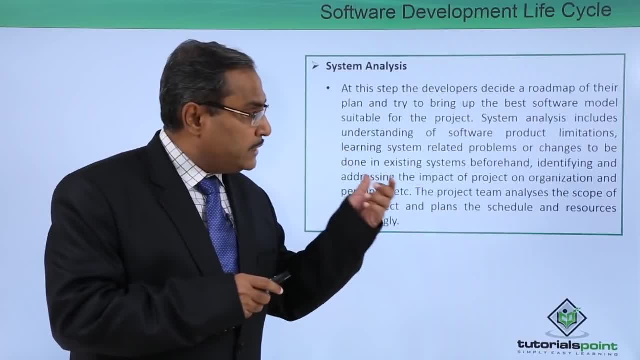 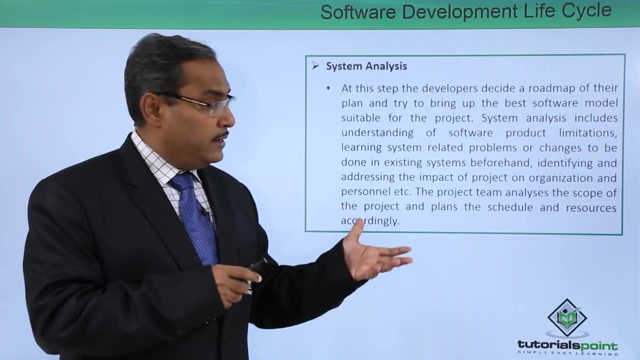 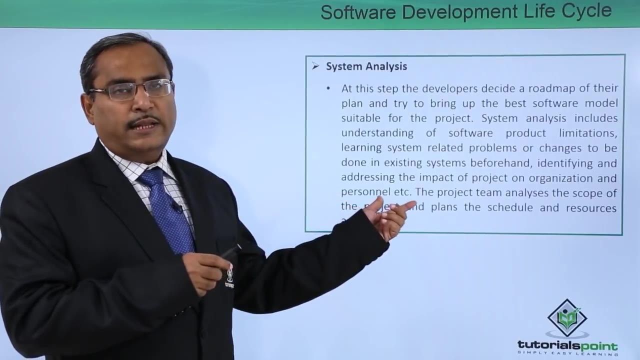 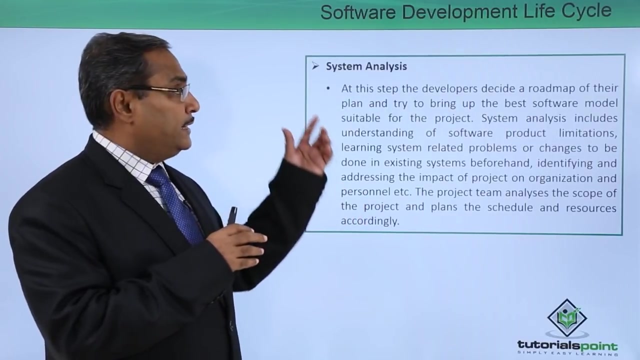 includes understanding of software, product limited simulations, learning, system related problems or changes to be done in the existing system beforehand, and identifying and addressing the impact of the project on organization and personal, etcetera. so these are the different steps. are different points to be noted, points to be taken care of in case of system analysis? that means, what are the different limitations? 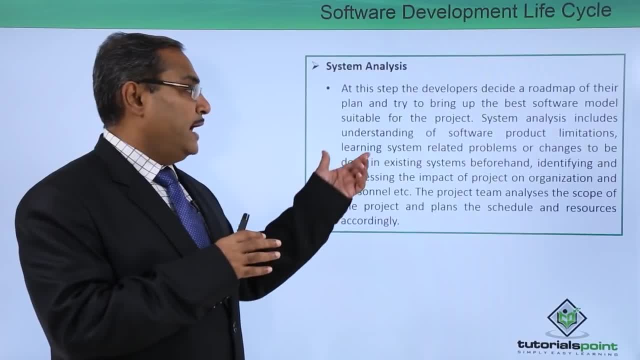 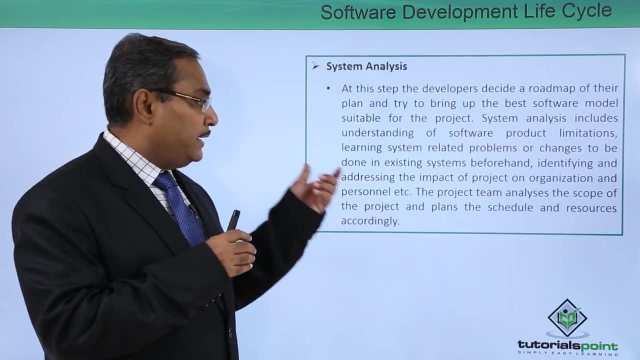 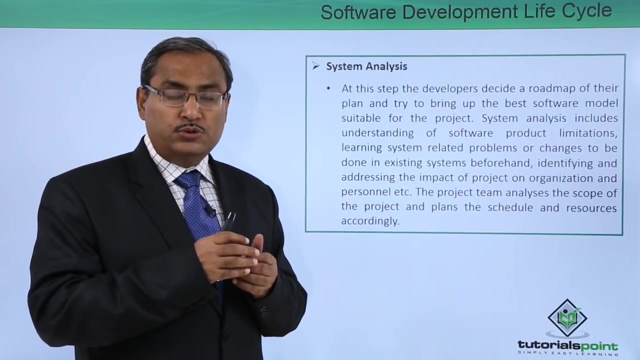 of the existing existing software, the understanding of that and then learning system related problems or changes to be done in the existing beforehand, and identifying and addressing the impact of the project on the organization and personnel who are going to use these softwares. So all these things are to be analyzed in this system analysis phase. 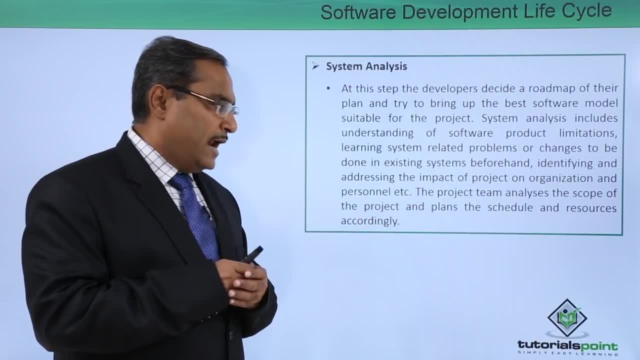 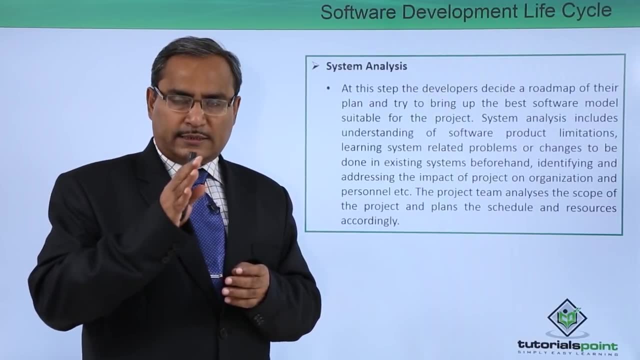 The project team analyzes the scope of the project and plans a schedule and resources accordingly. So what will be the plan? in which way? what are the different tasks and activities to be carried out and in which sequence will they be carried out in the in the sequential? 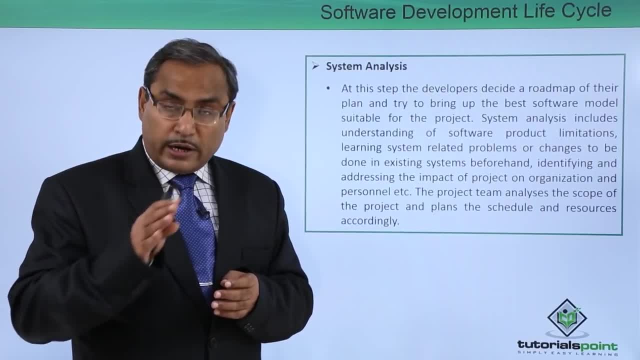 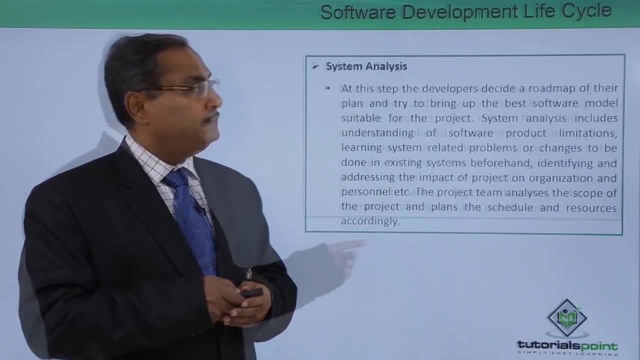 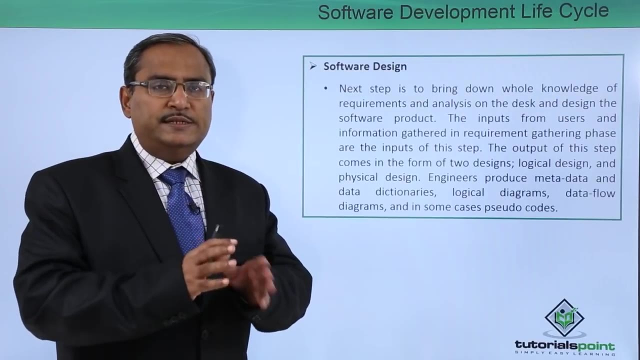 fashion or will they be carried out in the parallel and concurrent way? what are the different resources will be required? So all these things will be analyzed in this system analysis phase. After system analysis, we are going to discuss software design. The output of system analysis will be the input for this respective software design. 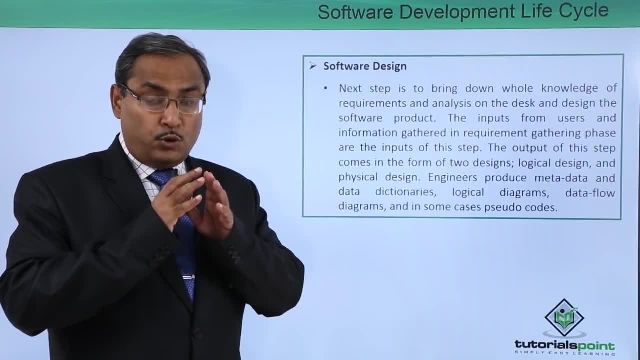 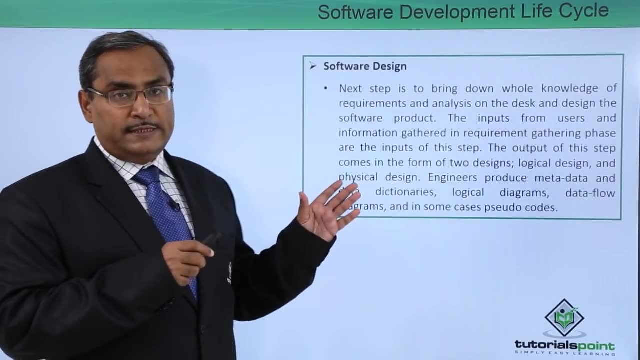 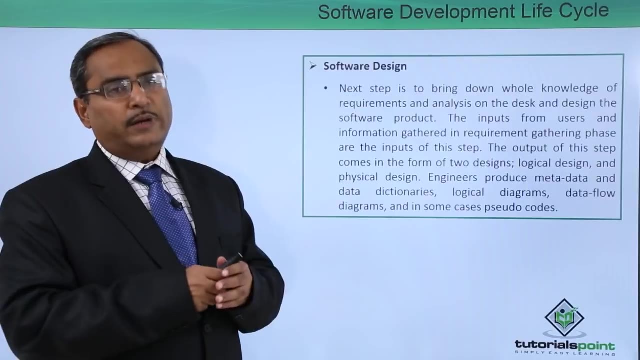 And all those analysis will be will be put, will be put in front of us so that we can design the software accordingly. And in this particular phase, we shall segregate our design in two, two types of: one is a logical design and the one is a physical design. 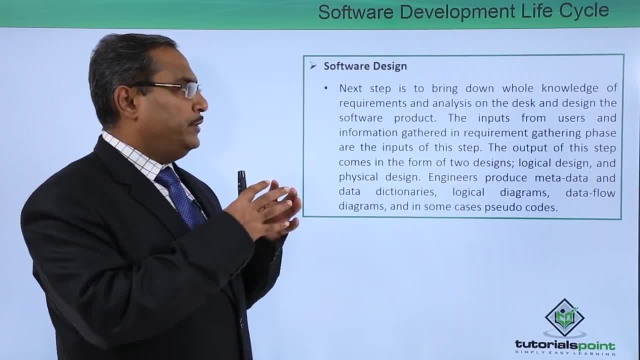 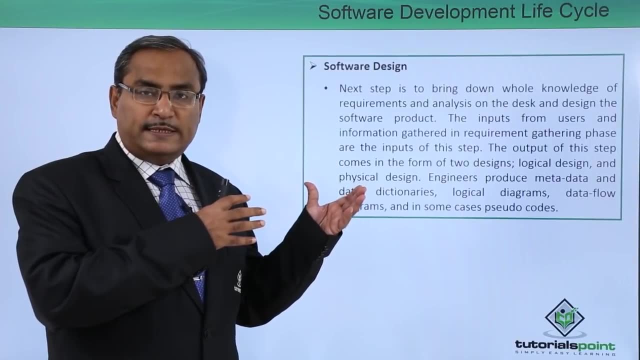 So next step is to bring down whole knowledge of the requirements and analysis on the desk and design the software product. So previous stage experiences will be discussed. Thank you very much. The data will be analyzed, will be taken care of in the software design. 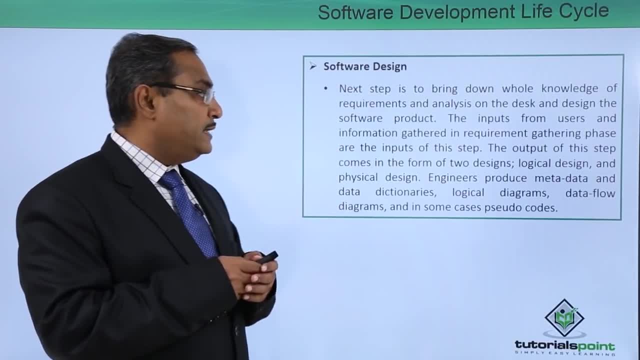 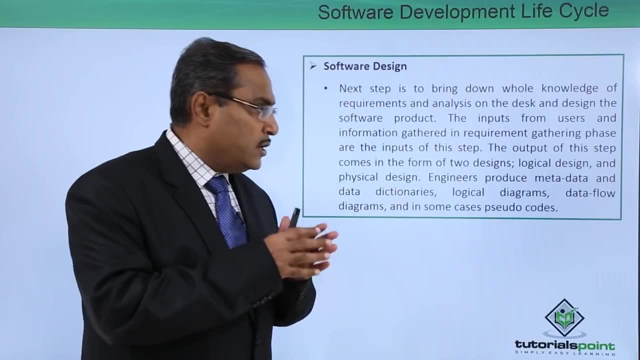 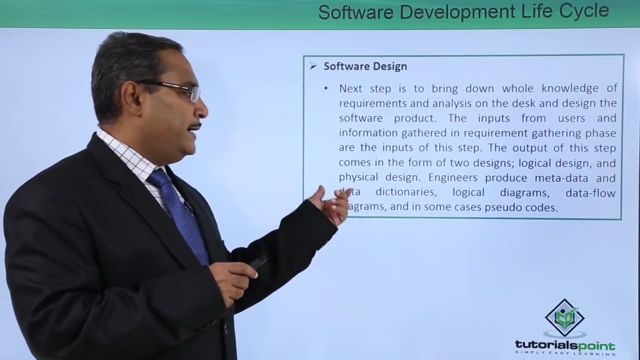 The inputs from users and information gathered in requirement gathering phase are the inputs of this step. The output of this step comes in for in form of two designs: one is a logical design and another one is a physical design. Engineers produce metadata and data dictionaries, logical diagrams and data floor diagrams, and 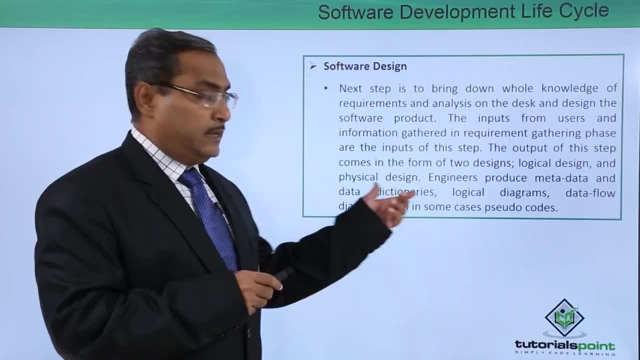 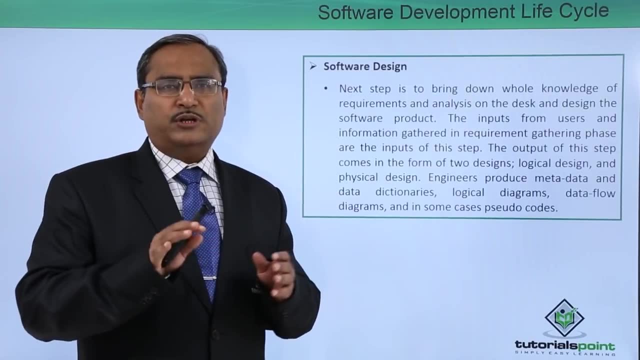 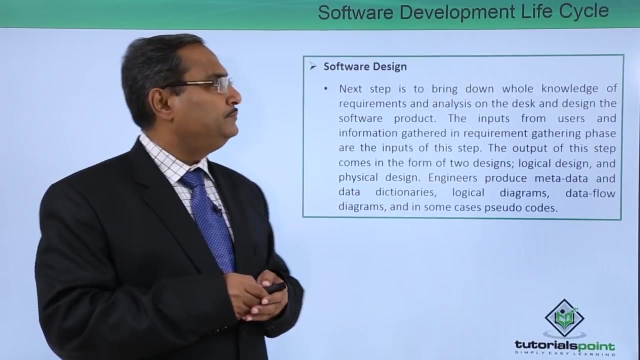 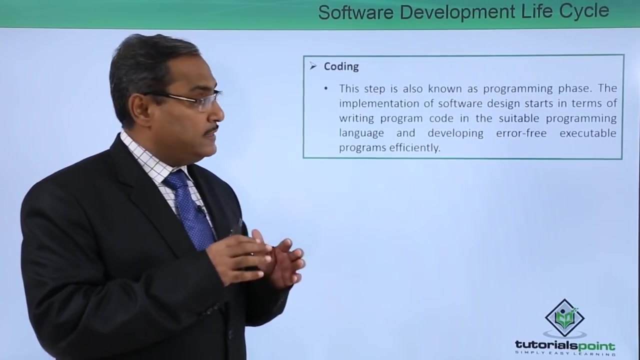 in some cases, pseudo codes For this respective defined type, different types of diagrams and different types of pseudo codes. we are having separate videos. please watch all of them. and those diagrams and this pseudo codes will be used in our software design phase. Next one: we are going for coding. this step is also known as the programming phase. 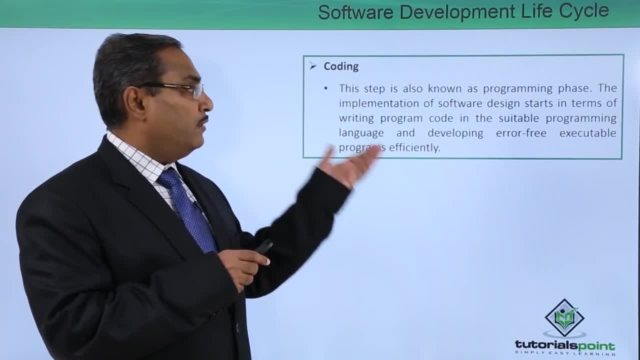 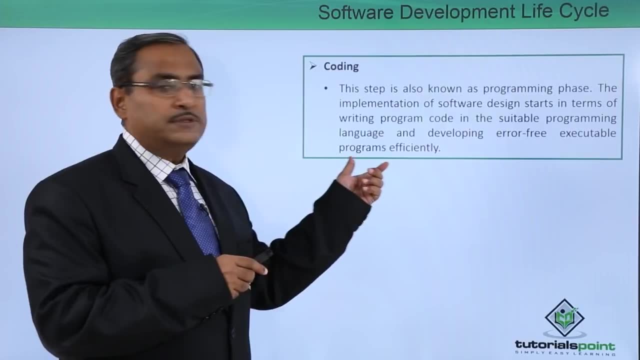 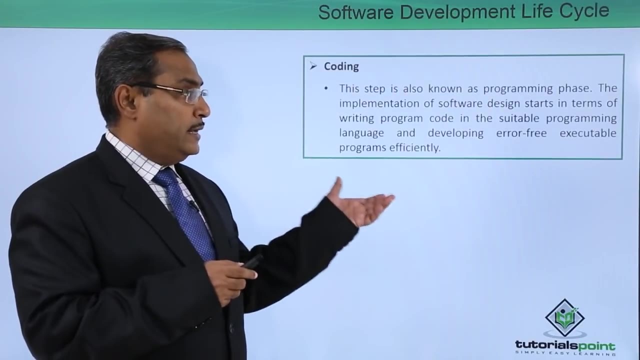 The implementation of software design starts in terms of the writing program code in the suitable programming language and developing error free executable programs efficiently. In this coding, obviously, you are also doing the simultaneously debugging of the of the code So that we can get some error free executable code which can implement the intent and purposes. 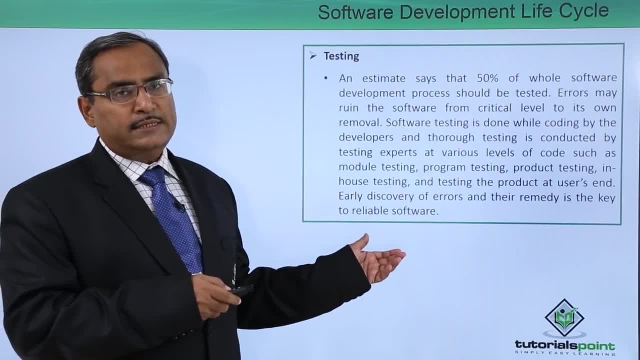 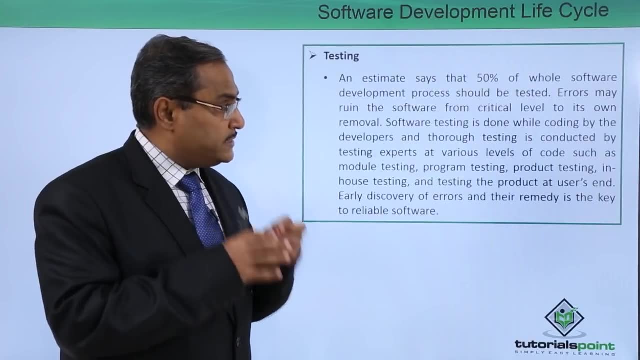 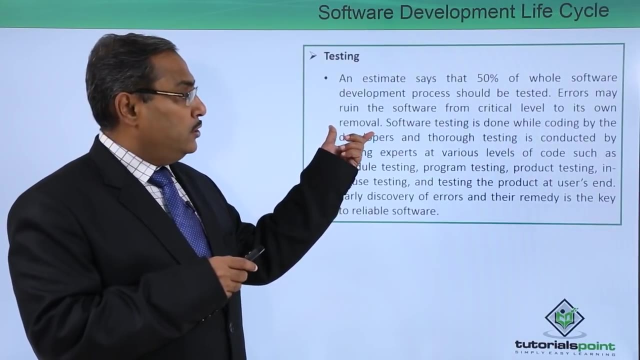 of the software. Next one: we are having this testing. An estimate says that 50 percent of the whole software development process should be tested and errors may ruin the software From critical level to its own removal. So that means errors are to be removed thoroughly. 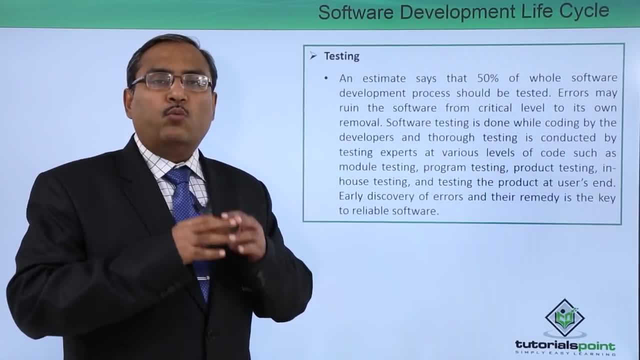 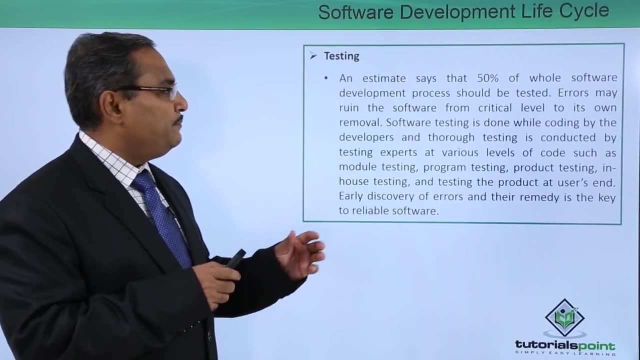 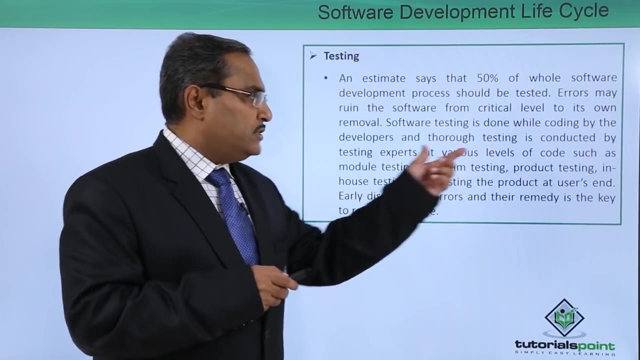 So that the software will be reliable and people can work on that. So that is why we should give our emphasis, very heavy emphasis, on this testing phase. Software testing is done while coding by the developers, and thorough testing is conducted by testing experts at various level of complexity. 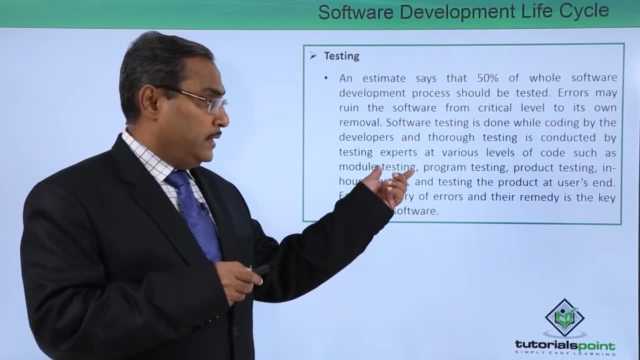 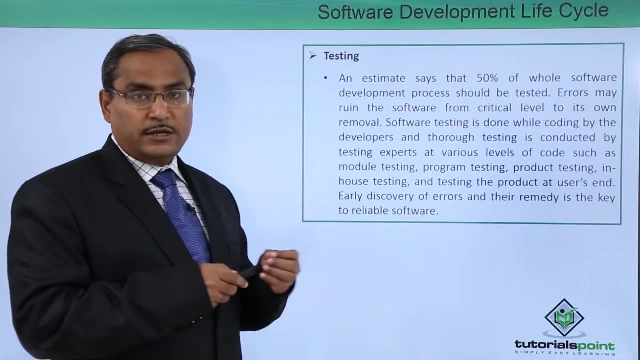 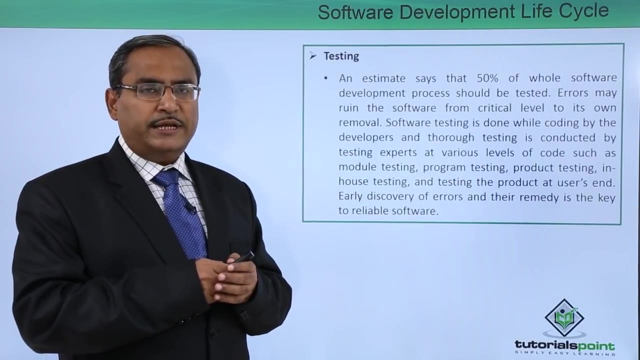 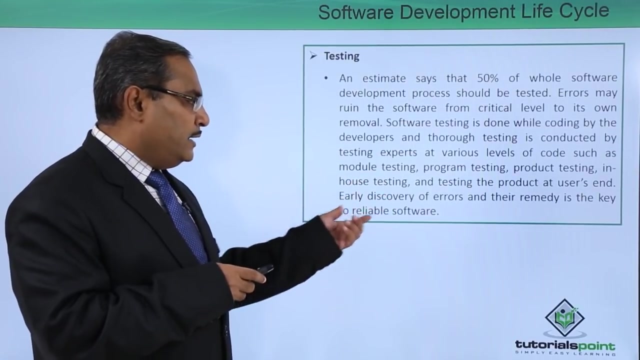 So there are different kinds of testing are possible, where having a separate chapter in our tutorial on the software testing you can watch them there. we have discussed all this testing method in do further details. Early discovery of errors and their remedy is the key to reliable software. 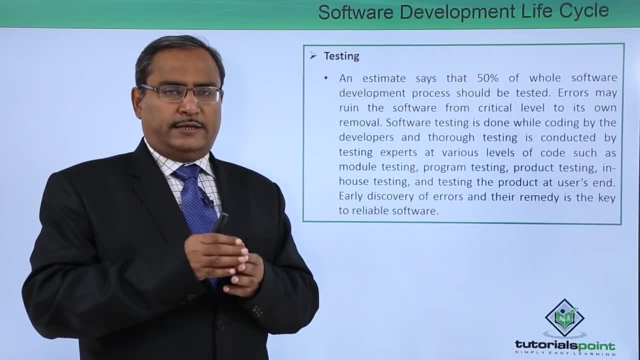 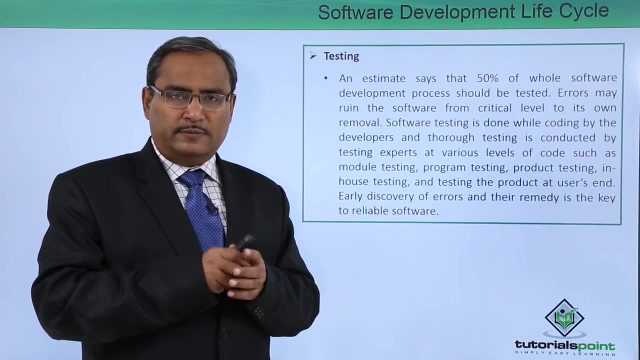 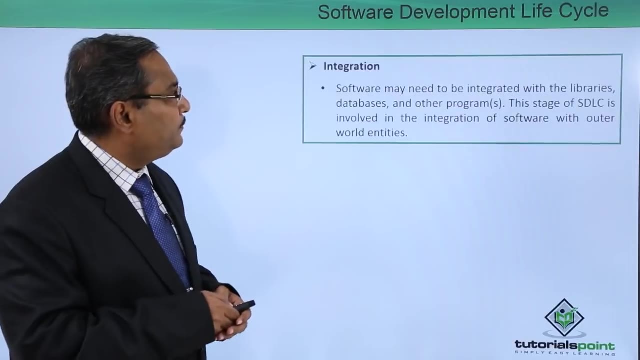 Whenever errors will get detected, if it it has got detected in the early stage of the software development, it will be less costly. but when it will get detected at the later stage of the software development then obviously it will be a very costly affairs for us. 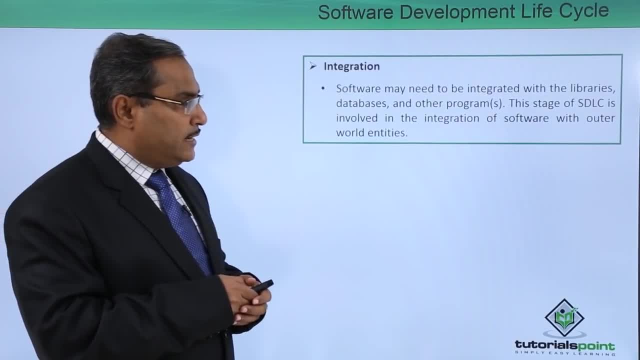 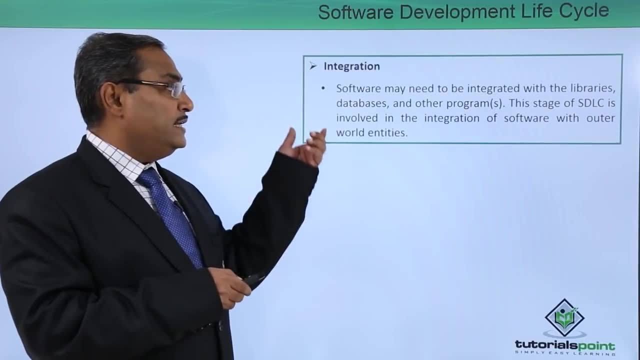 Next one is the integration. So software may need to be integrated with the libraries, databases and other programs. and this stage of SDLC is involved in software development. So the software may need to be integrated with the libraries, databases and other programs. 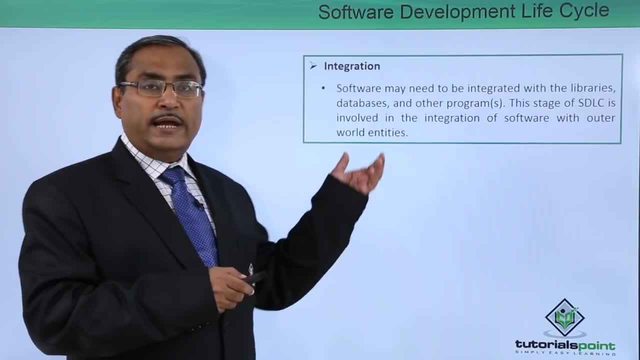 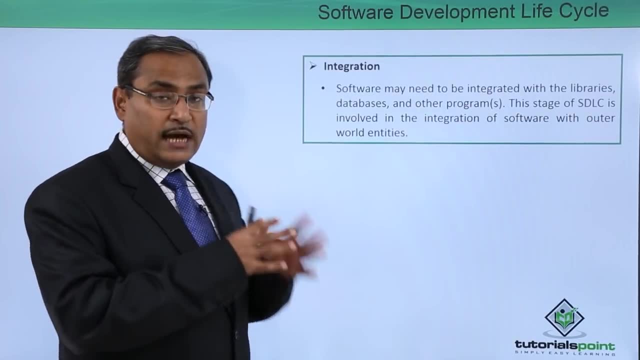 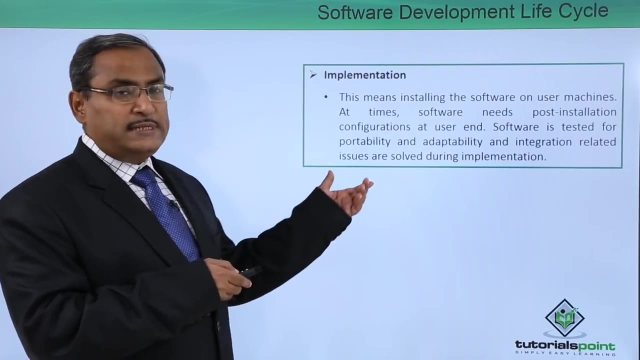 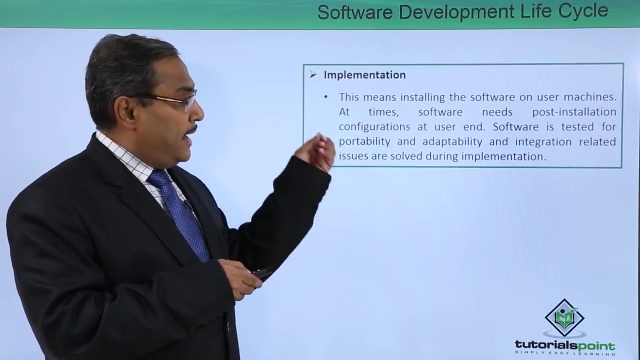 So all these things are to be integrated. So all these things are to be integrated so that the software can run and can give us the Influence lan log. Second one is the implementation. This means installing the software on user machines. at times the software needs post. 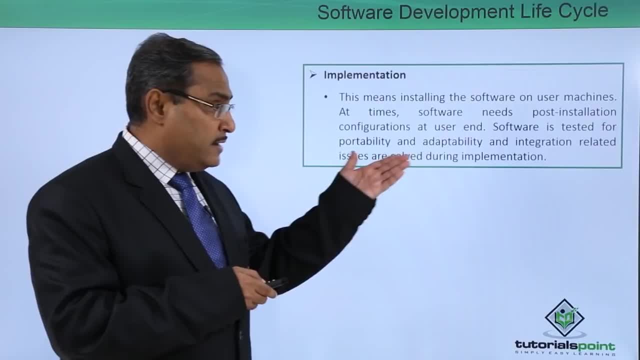 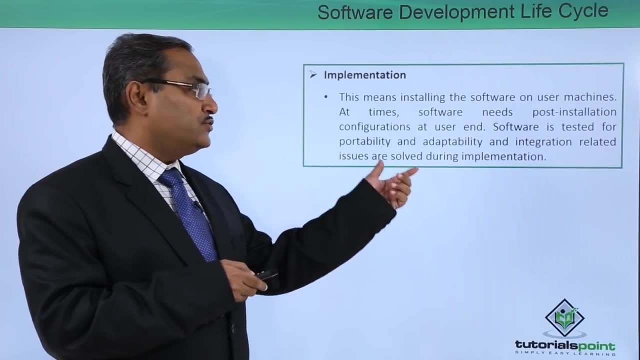 installation configuration at the user end. Now, in addition to it, everything else inside the point is 100% free. The components contain a set of by controller, cart and other devices, except for the. basically, software is tested for portability and adaptability, and integration related issues are solved. 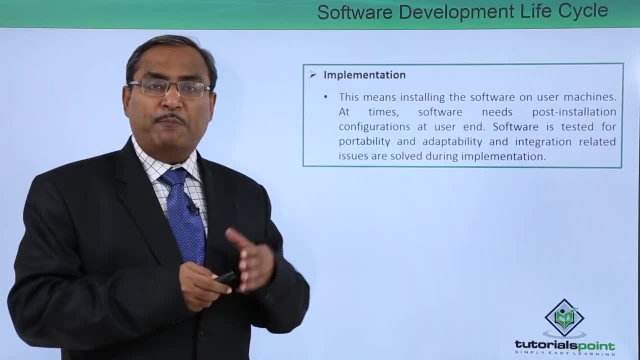 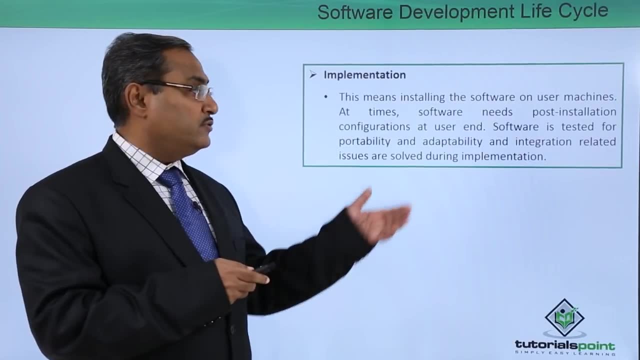 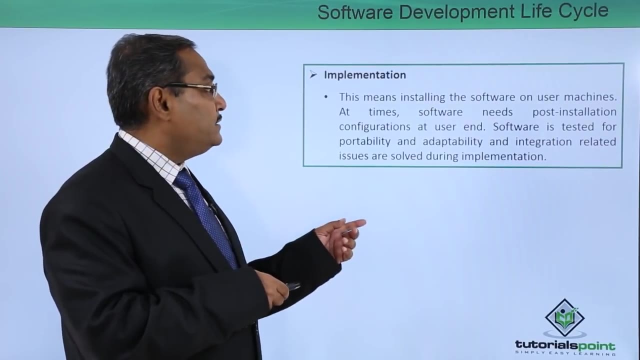 during this implementation. So now the software is going to get implemented, and during this implementation we are having some challenges like the we can check the portability of the software, the adaptability of the software and integration related issues, So this is known as the implementation phase. 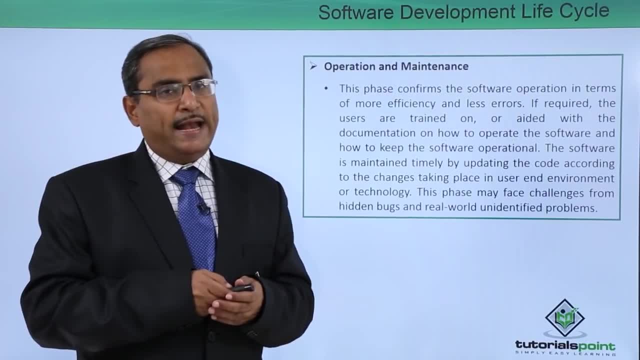 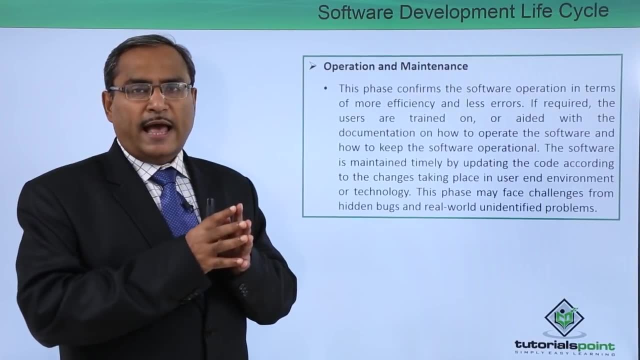 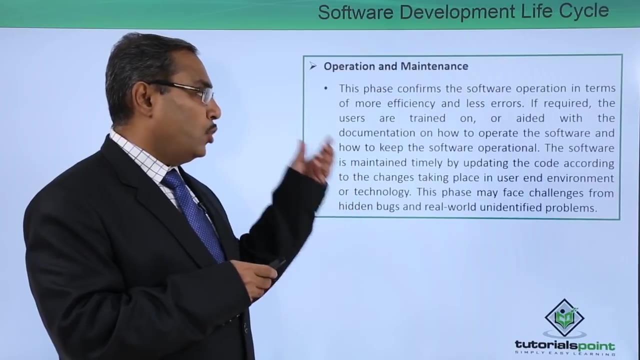 Now the next one is the operation and maintenance. So this phase confirms the software operation in terms of more efficiently and less errors. If required, the users are trained on or aided with the documentation on how to operate the software and how to keep the software operational. 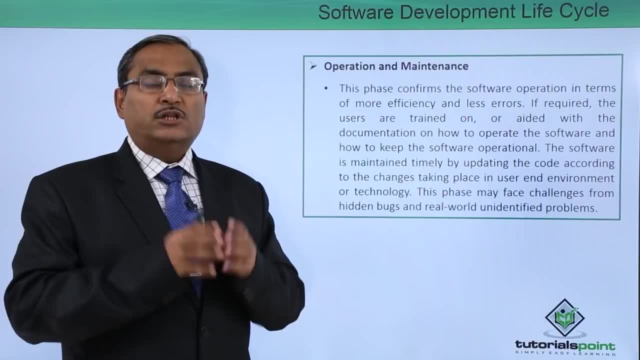 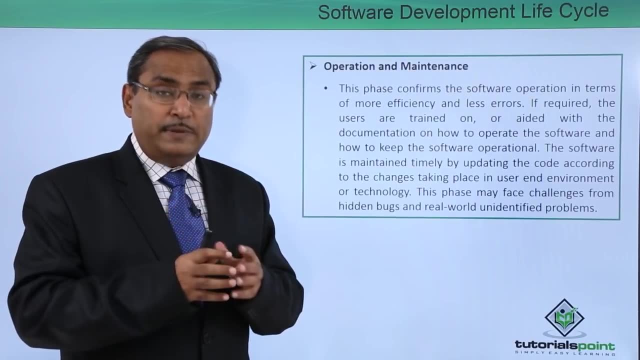 So, for this particular point, we should mention that the software should be user friendly, So the user can interact, Interact with the software in a very friendly environment, and we might be requiring some training to the user so that they can use it, use the software, in a fruitful way. 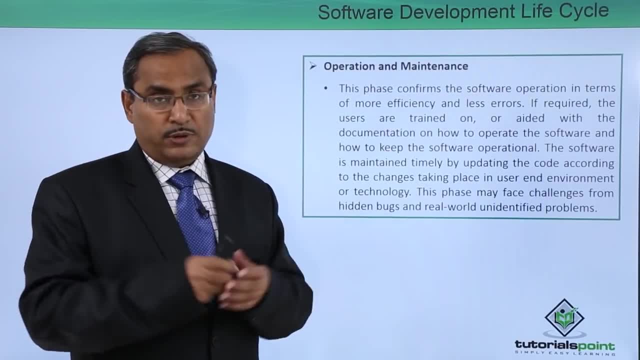 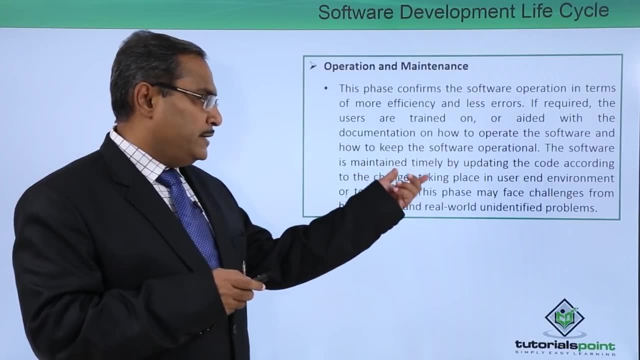 Some documentations can be given to them. some help files must be given to them. So that is why the user can get a very easy environment to work with the software. The software is maintained timely by updating the code according to the changes taking place. 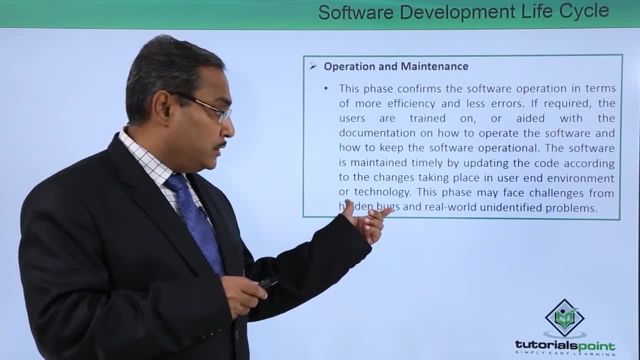 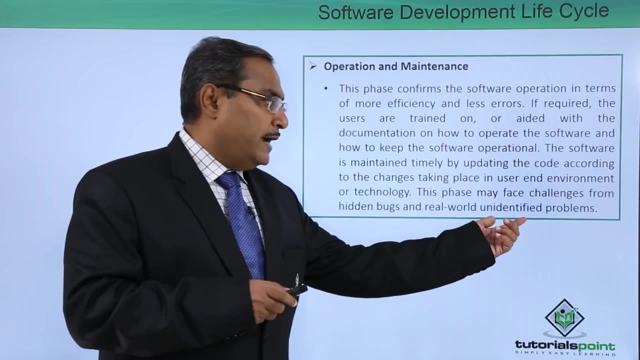 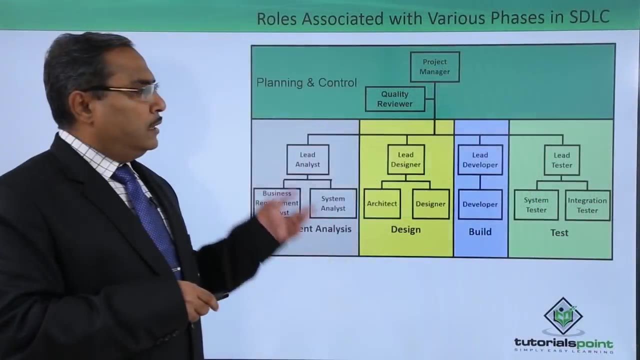 in user end environment or the respective technology. This phase may face challenges From the hidden bugs and real world unidentified problems, So this is known as the operational, operation and maintenance phase. Now, in this diagram, we shall discuss what are the different roles associated with various